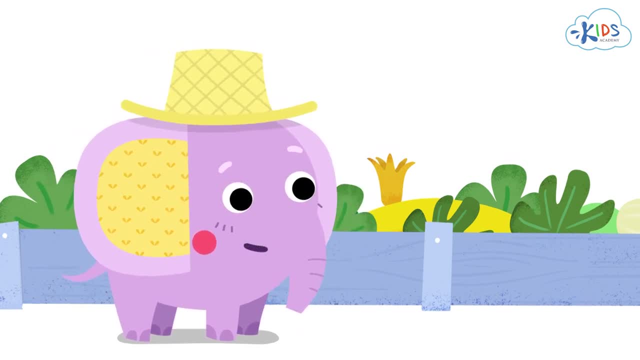 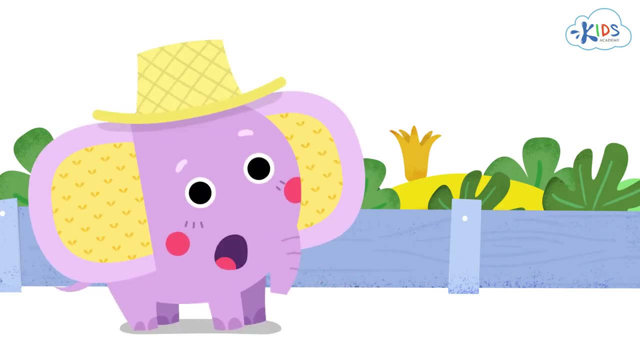 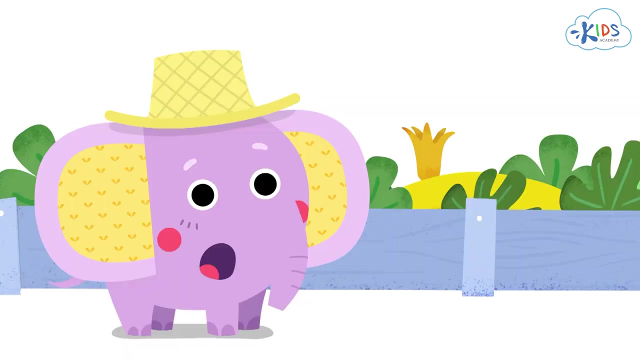 Wow, There are so many different squashes here. They're all ripe, except for the green ones too, right? No, Squashes don't change their color, But the riper ones are bigger in size, Got it? Then I'll collect the big squashes of any color. 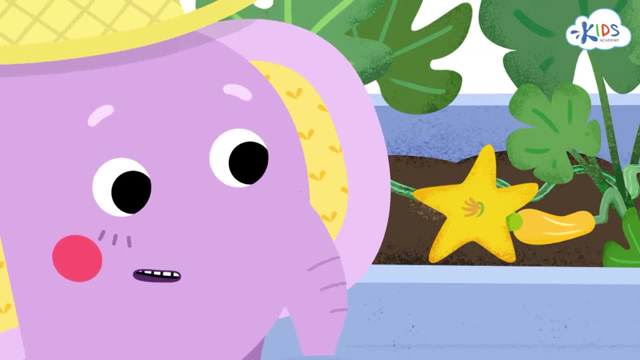 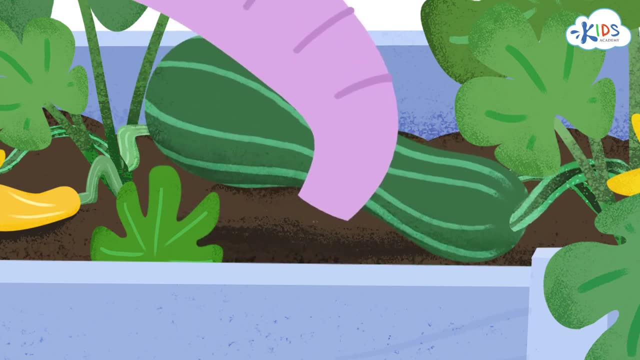 This yellow squash is so beautiful, but it's too small. Let it stay on the bed to get ripe. And this one is big And even though it's green, I'll pick it for my vegetable stew. This squash is big too, And I'll take this one. 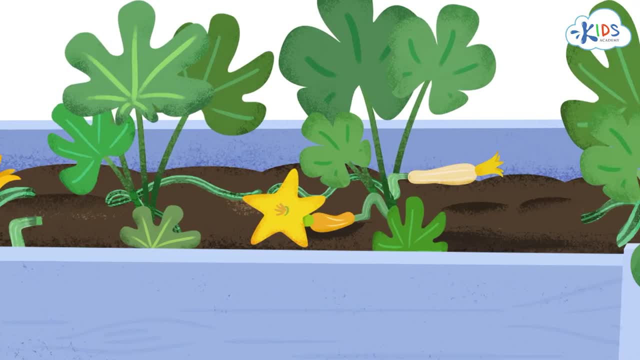 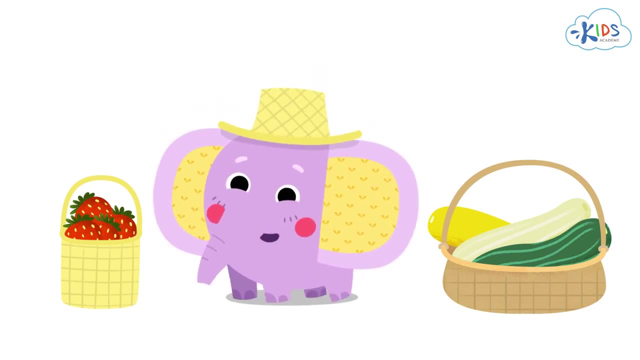 Awesome, Eddie. We can also say that you have just sorted the squashes by size. I've collected all the ripe strawberries and squashes. We'll make a great dinner from them, And we could do it because we know how to sort objects by color and size. 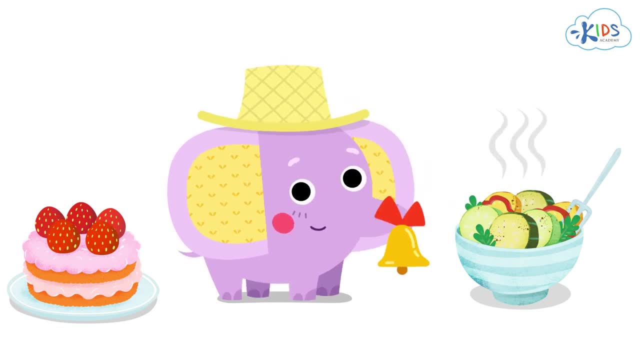 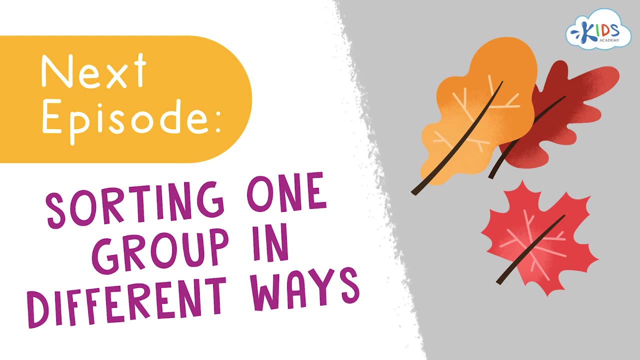 How can I sort the objects by color and size? Next time we'll talk about sorting the same group of objects different ways. See you soon.